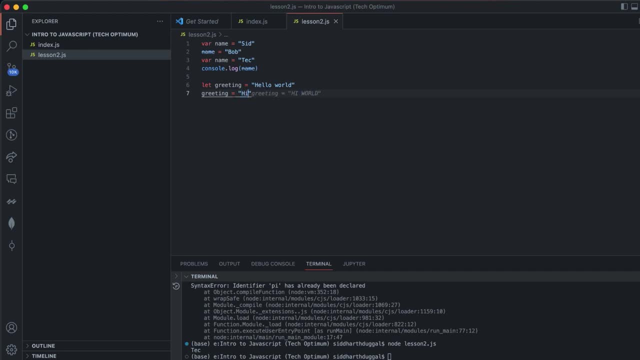 hi world by simply doing the variable name equals and then your value. The catch with let is that you cannot do let greeting equals by world because you will get this error cannot redeclare block scope variable greeting. So if you want to reinitialize a variable, you should. 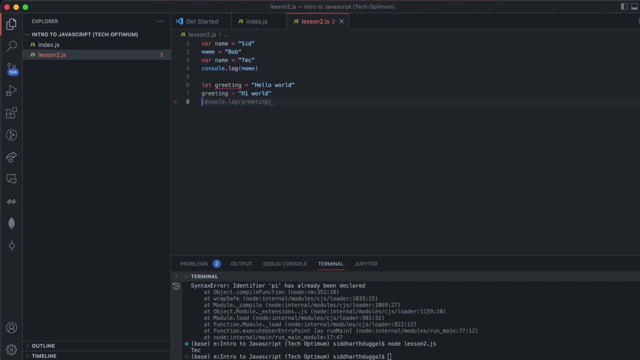 use the var keyword and not the let keyword. So let's go ahead and delete this. And let's go ahead and console log greeting and run this code. So let's go ahead and delete this. And let's go ahead. this code And, as you can see, it displays hi world, which was the last way I changed the. 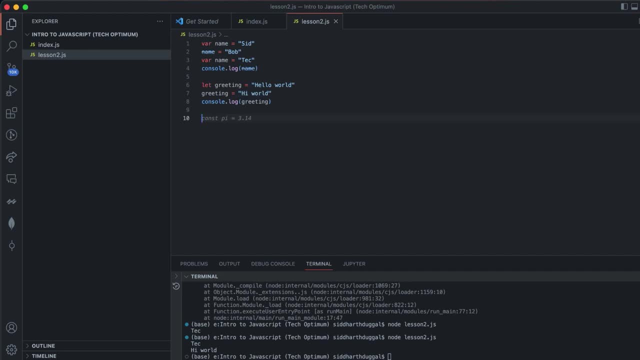 variable. So now let's take a look at the const keyword, which is the strictest way of declaring variables in JavaScript. So let's go ahead and set pi to 3.14 by doing const, pi equals 3.14. And then if we try changing the value of pi to 3.15, it'll declare an error. Let's go ahead and console. 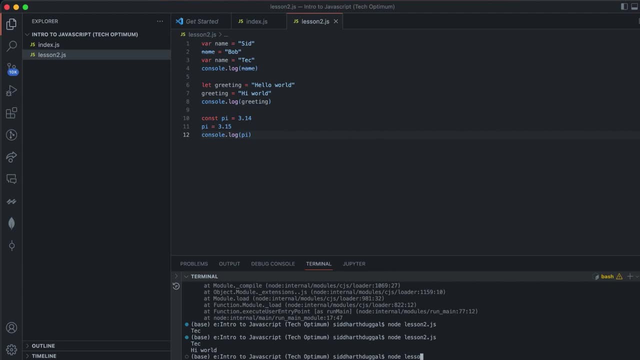 log this And, as you can see, it gives an error because you cannot reassign a value to a const variable And if you try reinitializing it, like you did with the var variable or the let variable, it'll also give. 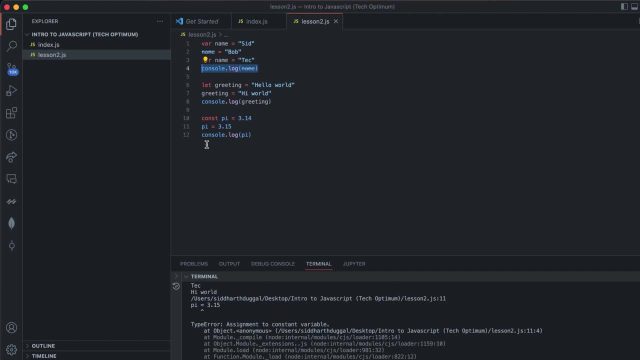 an error because it is a const variable And once you set it, it cannot be changed. So understanding the difference between var, let and const is crucial, as they help you decide how to label your variables. So now let's take a look at the second part of this lesson, And I'll see you in. 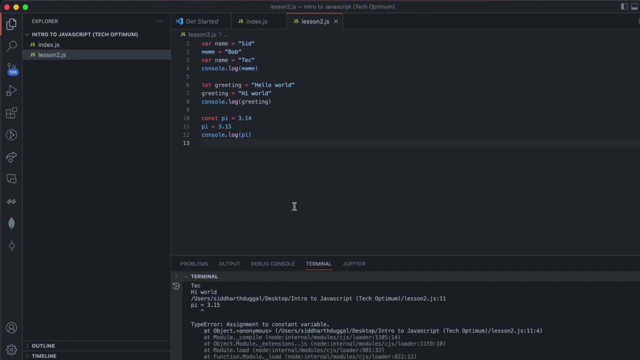 the next lesson, which is exploring different types of data types in JavaScript. So let's take a look at numbers first. There are two main ways of declaring numbers. So let's go ahead and declare a number one of five- and no need to put quotation marks around five, because it is an integer- And let's go ahead. 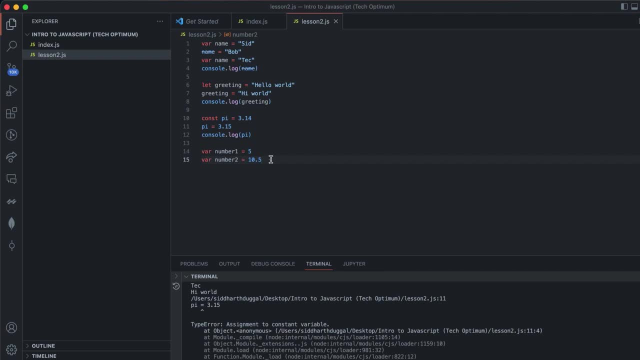 and declare a float by doing 10.5.. A float simply means it is just a decimal. So now let's take a look at another way of declaring variables. in JavaScript, You can simply do var string. one equals quotation marks. Hello, And this is the only way of declaring a string, by doing these. 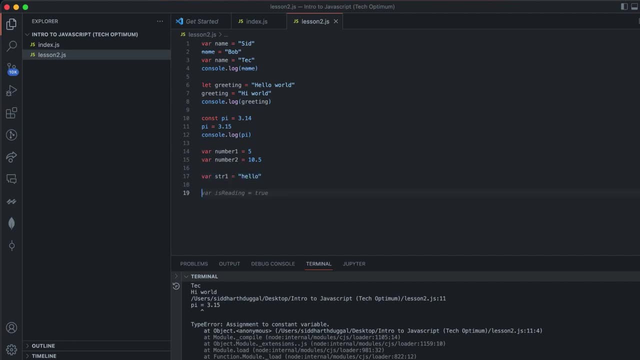 quotation marks. Another data type in JavaScript is booleans. So let's go ahead and set is reading to true and that. And yet again you do not need quotes around- true because it is a boolean expression. And let's do. var is sleeping, equals false And boolean expressions only have two. 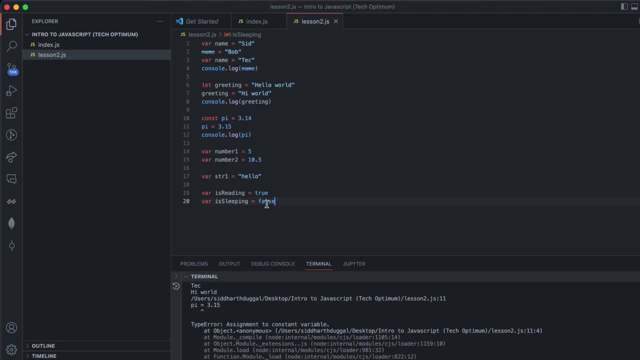 values: true or false, nothing in between, or more. These variables are often used for conditional testing, which we'll get into later in this course. So now let's go ahead and combine the concepts of variables and data types. One cool thing that you can do in JavaScript is concatenate variables or strings or numbers together. So let's go ahead. 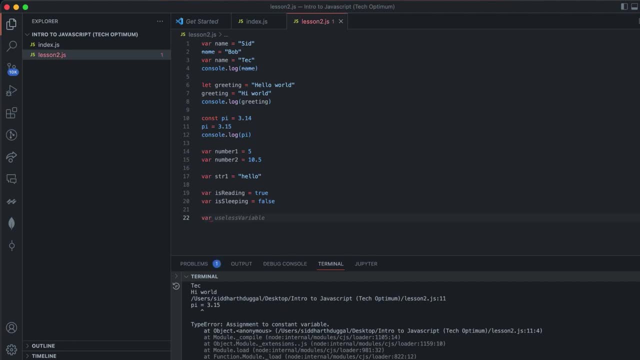 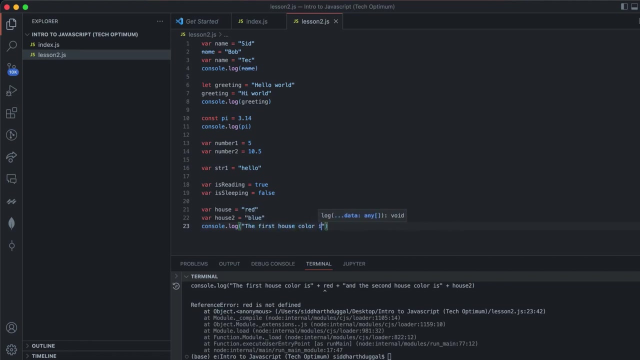 and do this. We can simply set var house equals red. We can make another house var house. two equals blue. So let's go ahead and concatenate both of these variables in a console dot log statement. Let's do console dot log quotation marks. The first house color is space house. 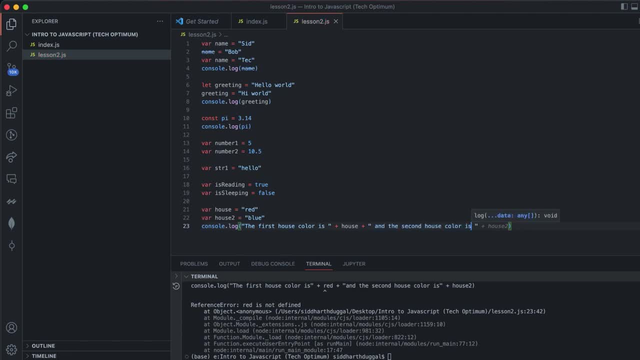 And the second house color is house two. And so if we go ahead and run this code, you'll see it says the first house color is red and the second house color is blue. By using this plus operator, you're able to combine these strings along with these variable. 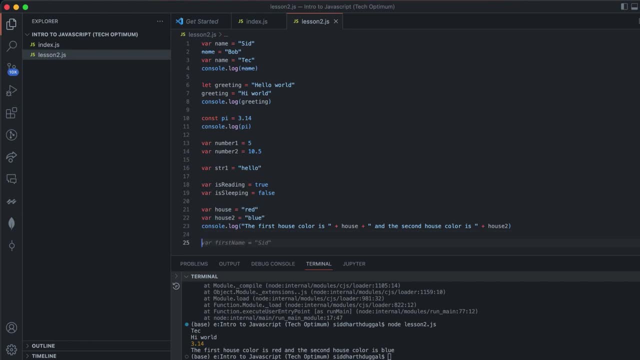 strings, which is a pretty neat feature in JavaScript. Let's practice this with numbers, instead of concatenating it using strings. Let's simply add it. So let's do: var number 10 equals 10 and var number 20 equals 20.. Let's go ahead and console log these, So the output: 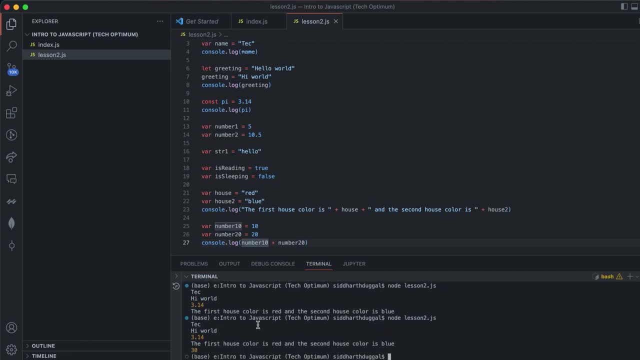 should be 30. So let's go ahead and run this code And, as you can see, displays 30. So that's it for lesson two. be sure to be familiar with variables and data types, as it sets the foundation for JavaScript. In the next lesson, we'll look at control structures which allow your code to make. decisions and repeat actions. So I'll see you next time and I'll see you at class. Bye for now. Y'all take care and I'll see you again next time. Thank you for watching. Thank you bye, So I'll see you then.